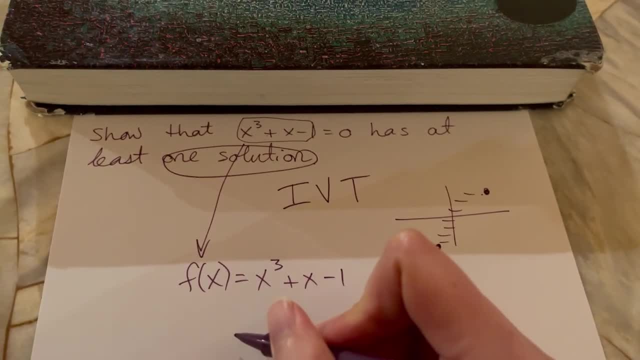 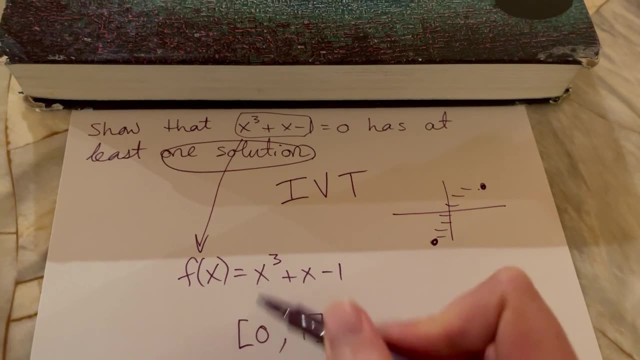 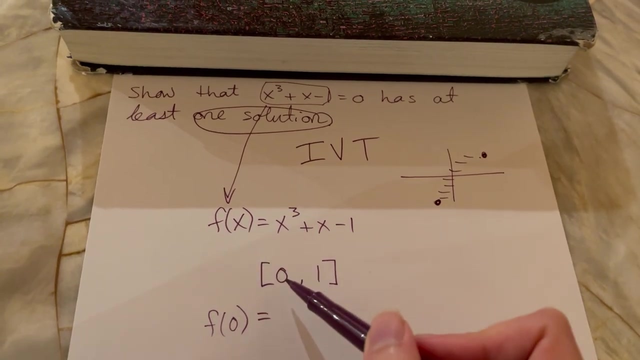 try a different interval. So for instance, you could try the interval zero comma one maybe and see what happens 0,1, maybe. and see what happens 0,1, maybe and see what happens When you plug in zero and when you plug in one. what do we get for a function? height at zero. 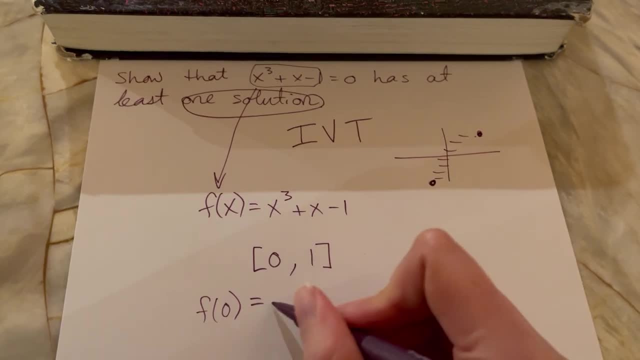 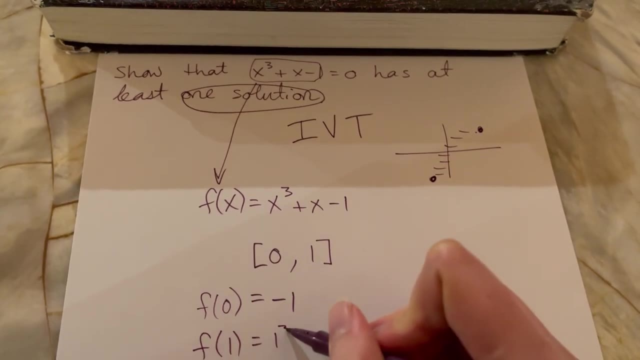 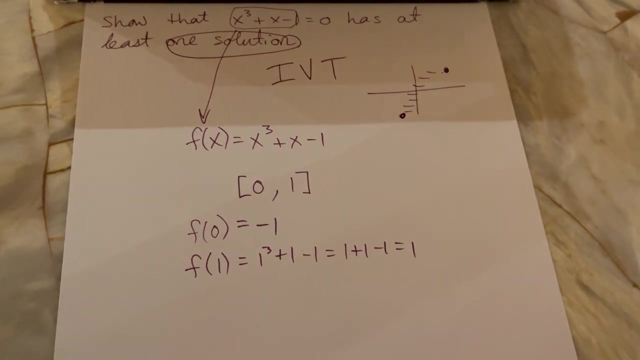 Well, we get zero cubed plus zero minus one, And if we plug in one, we get one cubed plus one minus one. We get one plus one minus one and we get one for our answer. Okay, so that actually works If we started with our function. 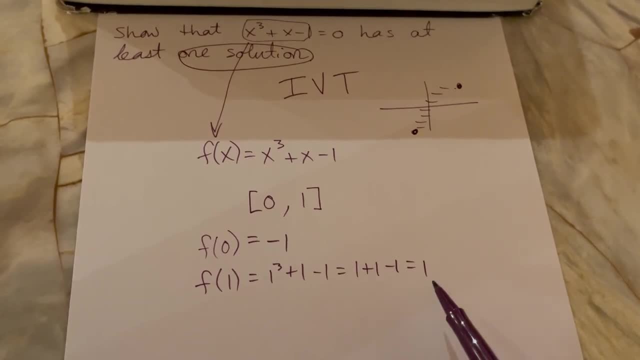 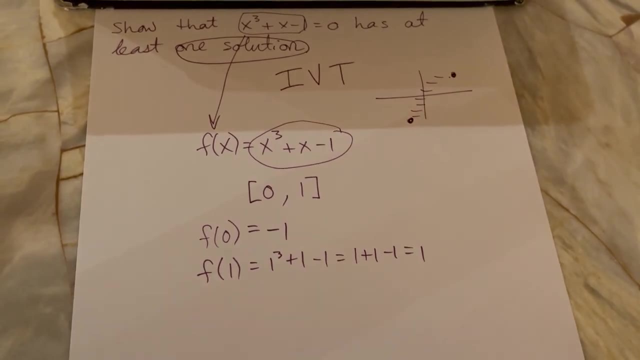 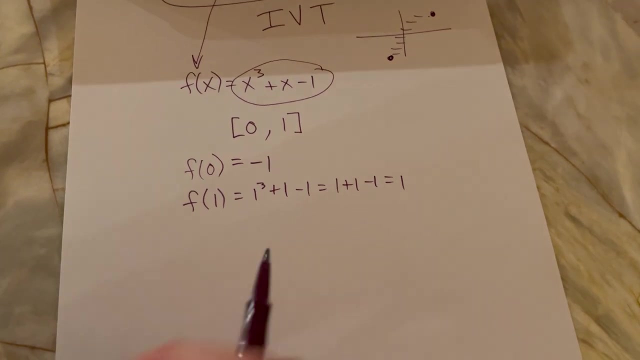 height being negative and we ended up with a positive function- height. then, because this is a continuous function, by IVT this function equals zero somewhere in between here. So what you could say for your final justification, if it asks you to justify. 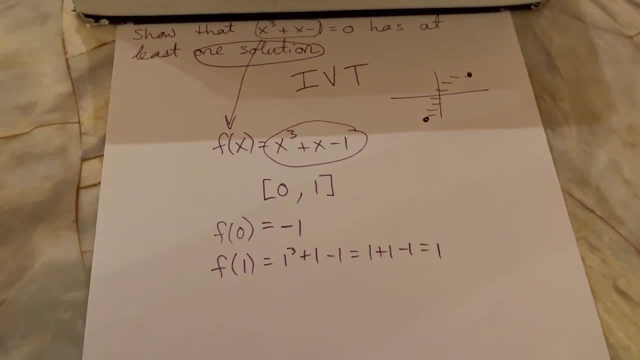 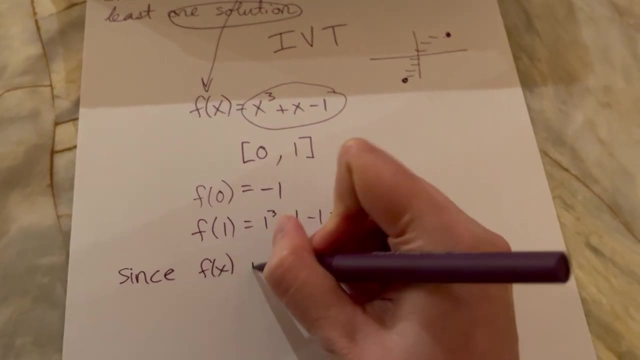 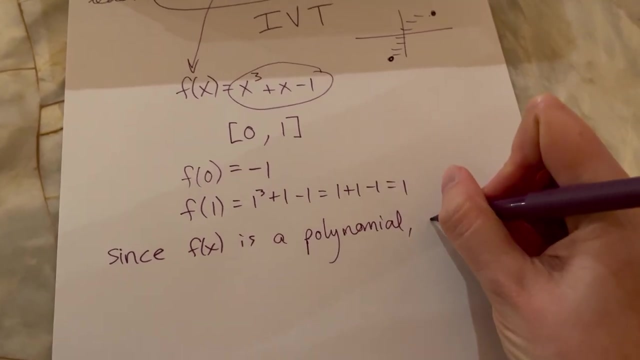 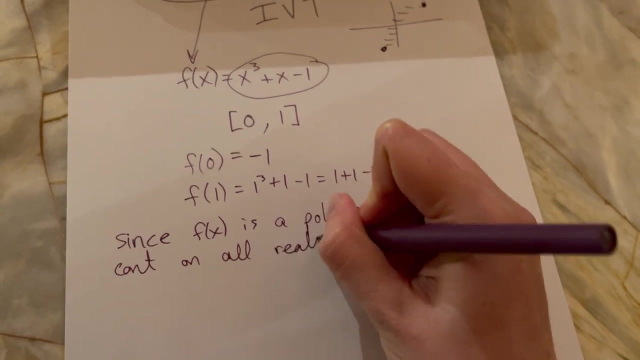 your answer and it wants a nice solution with reasoning and theorems. you could say: since f is equal to zero, you could say: since f of x is a polynomial, it is continuous on all real numbers. so we can apply. 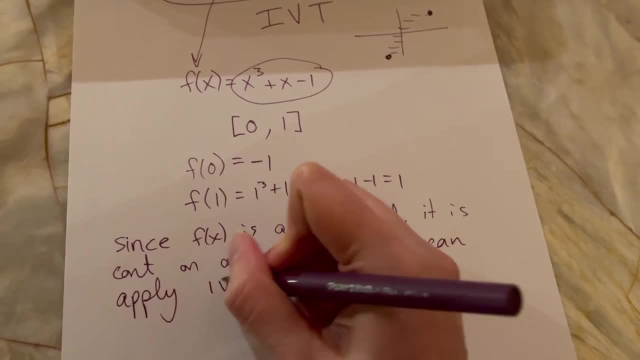 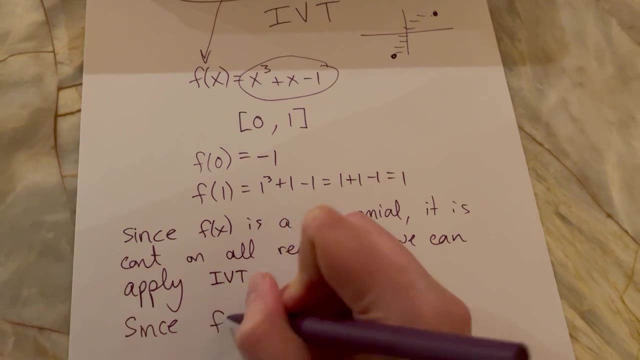 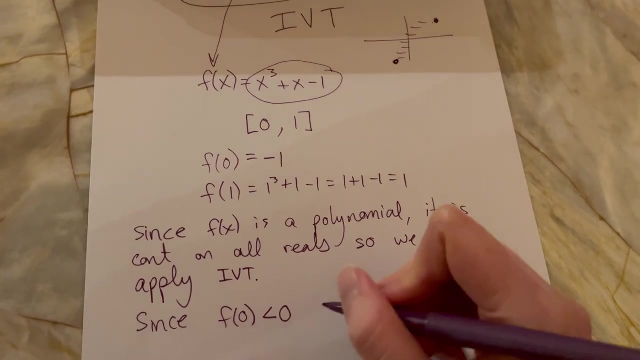 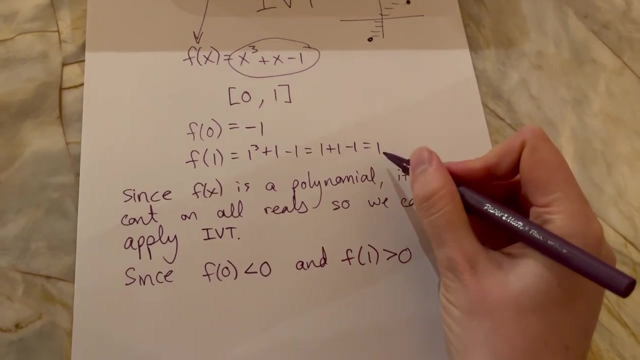 the intermediate value theorem. And then you would say: since our left end point f of zero was a negative height, so less than zero, and then later our right end point height was greater than zero, it was positive one. that means: 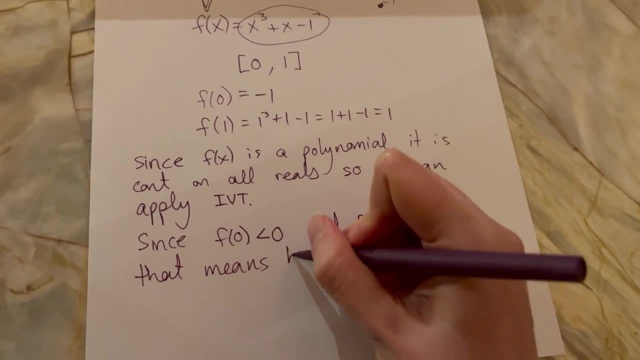 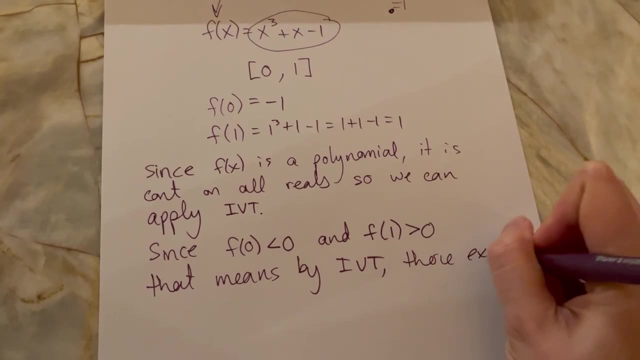 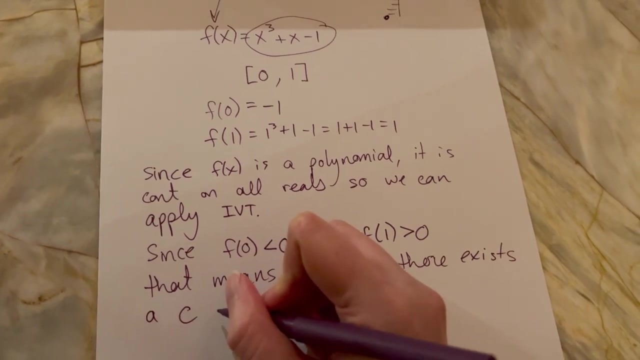 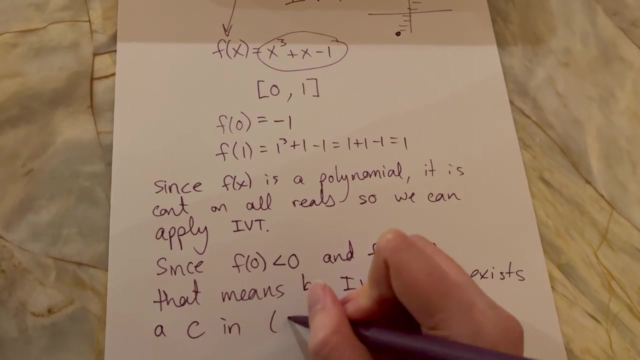 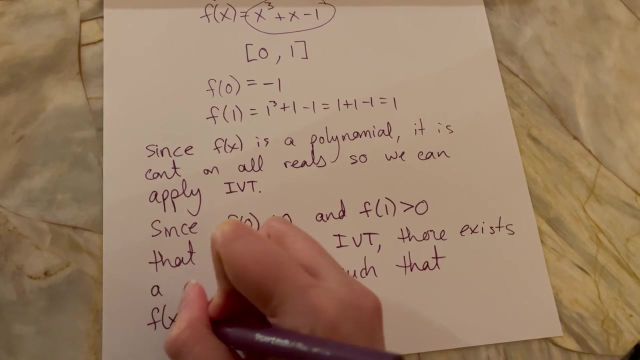 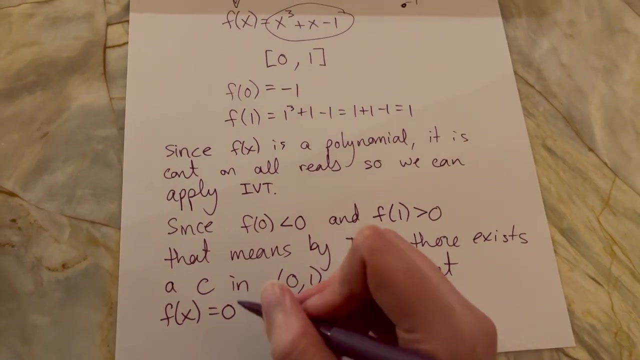 by IVT. there exists a, c. Usually they call them c. it's an x value, c in the interval zero, comma, one such that f of x has a height of exactly zero. Okay, and since that was actually the original solution, we can say: